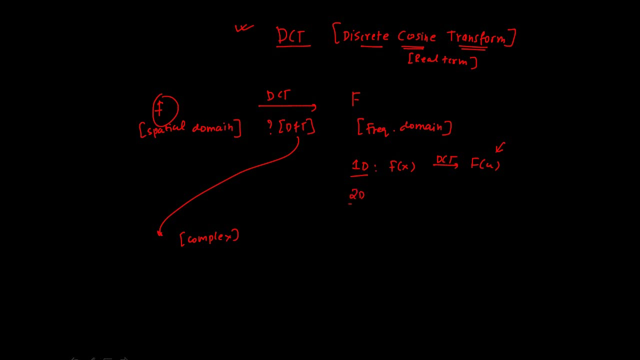 frequency domain of an image. Suppose I have the two dimensional image. Now it can be F of X, Y, any, any pixel value it can be. I'm taking in general one function: F of X- Y. If I apply the DCT here now, I will get capital F of U? V. So this is my basic idea. I have to transform this image into the frequency domain. Now the next question is: how can I apply the DCT and I can achieve this? capital F of U? V. So this is my basic idea. I have to transform this image into the frequency domain. Now the next question is: how can I apply the DCT and I can achieve this? capital F of U V. 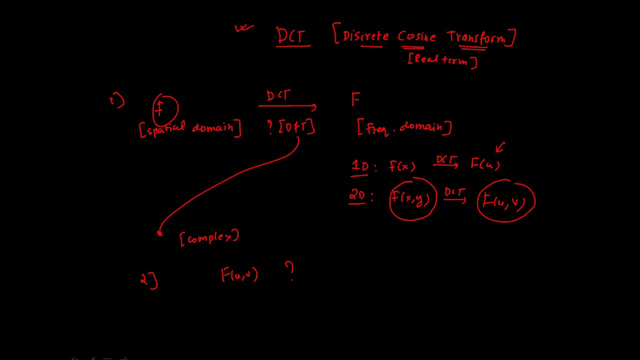 v correct. so let's see how we can find capital f of u, or let's say capital f of u, comma v, because this is one dimensional, this is two dimensional. now the answer for that is pretty simple. if you have to find f for one dimensional, it would be c into original image. if you have to find capital f, 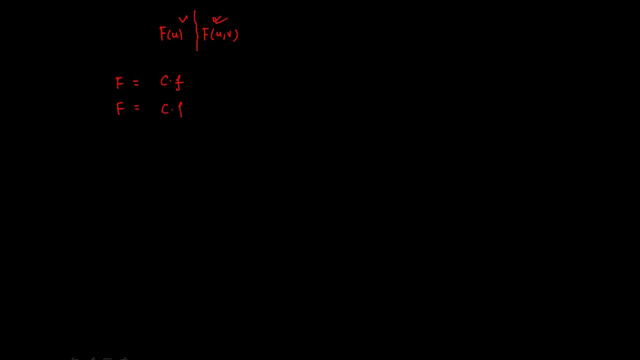 for two dimensional image, it would be c into original image, into c transpose. now your question might be: what is this c? so c stands for discrete cosine, or let's say cosine transform matrix, so cosine transform matrix. so the formula of c of u comma v is equal to root of 1 by n, and when u is: 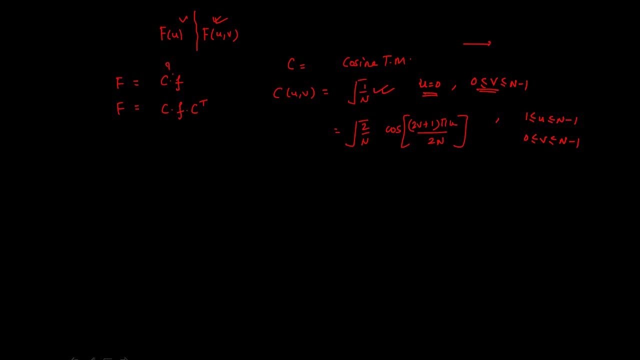 0. that is for the first row, and v changes from anywhere between 0 to n minus 1. so if I have this matrix, let's say this is the u side, this is the v side. so u is equal to 0, means the first row, we are talking about the first row, and v can be anything like 0, 1, 2 up to n minus 1. 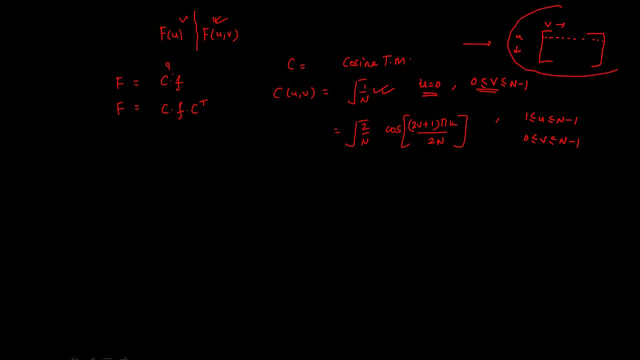 so I hope you are getting this point. we are talking about the c, that is the cosine transform matrix. so for the rest column, we have root of 2 by n into cos of 2v plus 1 pi u upon 2n and the range is this: from the rest of the part, the formula would be this, and for the first row, the: 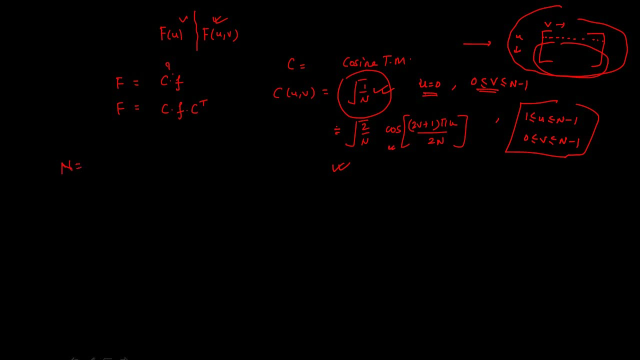 formula is root of 1 by n. so when we talk about the size 4, that is, n is equal to 4. let's talk about this c of u comma v. now here we write u correct, so it would be 0, 1, 2 and 3, because u. 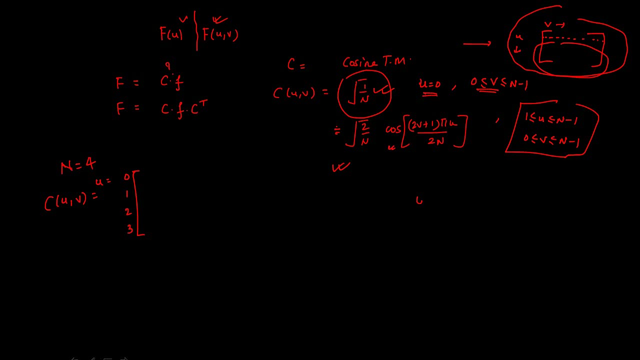 ranges from 0 to n minus 1. as you can see, the range for u and v is 0 to n minus 1. this is the complete range. so is writing here? so 0, 1, 2, 3 now to get the first row? what was the formula to get the first row? 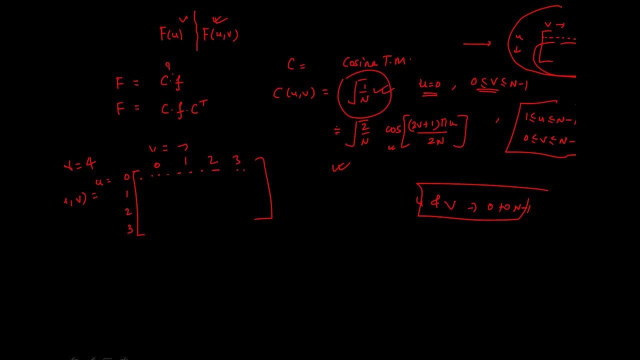 u is equal to 0 and v is equal to 0 to n minus 1, because n is 4 here. as you can see, n is 4, correct. n is 4 here. so the range here would be 0 to 3 and for that the answer is root of 1 by n. 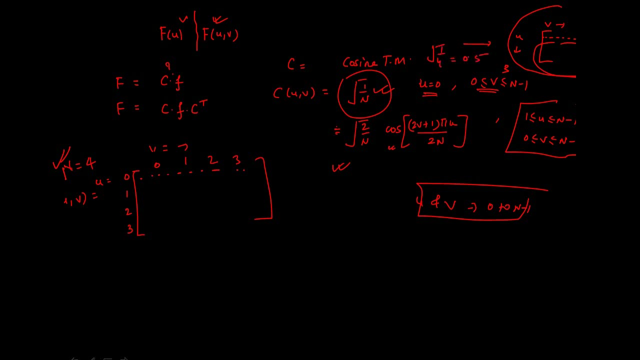 that is equal to root of 1 by 4 and that is equal to 0.5. so the first row we have 0.5, 0.5, 0.5, 0.5 and the rest part you can find using this formula and the trick to remember this. 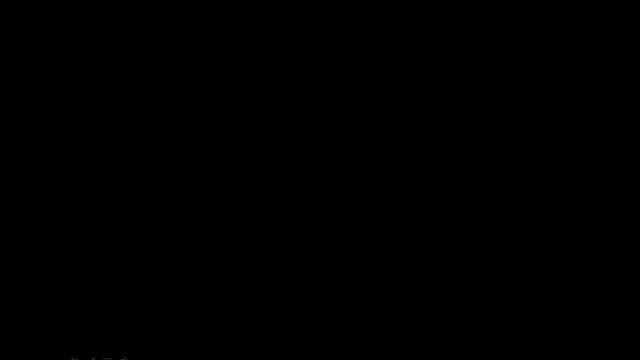 let's see in the next slide. so let's learn about the trick: how to remember c of u, comma v for 4 cross 4. now this is a pretty cool trick. let me draw this big. all right, so u is equal to 0, 1, 2. 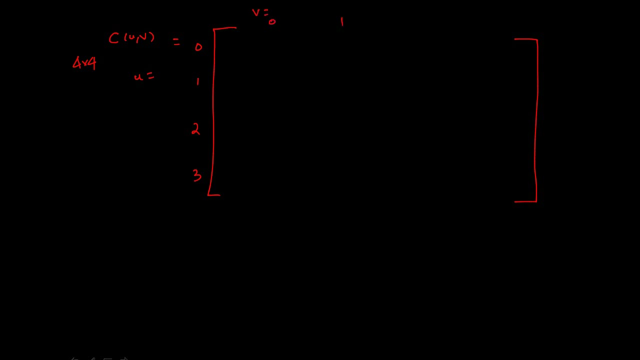 and 3. similarly, v is equal to 0, 1, 2 and 3. now the first column was simple, as you saw: 0.5, 0.5, 0.5, 0.5, because root of 1 by 4 is equal to 0.5. 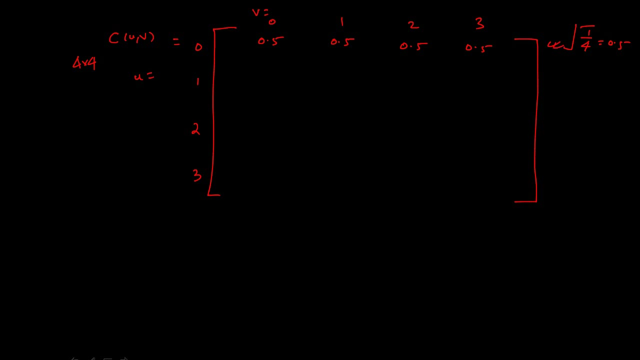 this was the first line of the formula root of 1 by n. for the rest, the formula was different and if you put 0, u is equal to 1 and v is equal to 0 in the second formula, then you will get the answer as 0.6. i have 5, 3, and if you put u is equal to 1, v is equal to 0 and v is equal to 0. 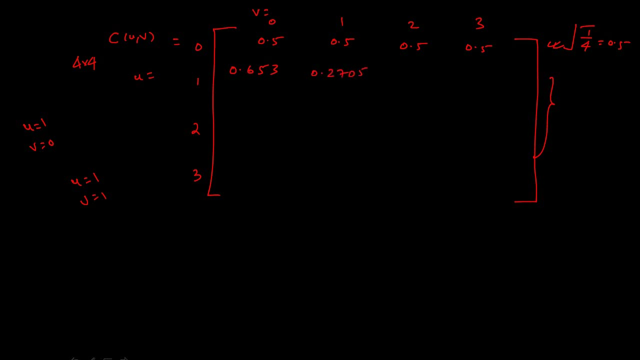 you will get 0.2705. now this is a pretty interesting trick. now the trick is for the row 2. the value remains similar to row 0, so it would be 0.5, 0.5, 0.5, 0.5. now why i draw this line? 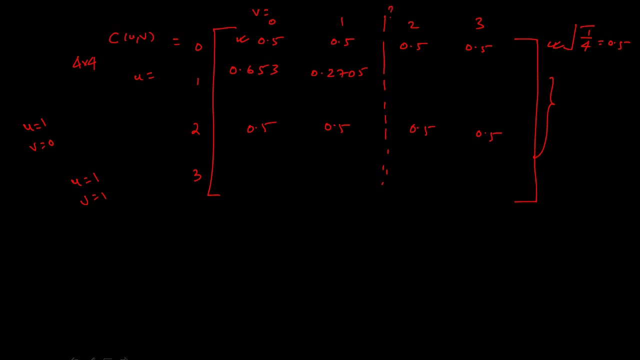 the reason for that is the value is like a mirror, so the value here would be same as 0.2705. the value here would be same as this: 0.653, so 0.653. now take this value and shift here, so the answer is 0.2705. 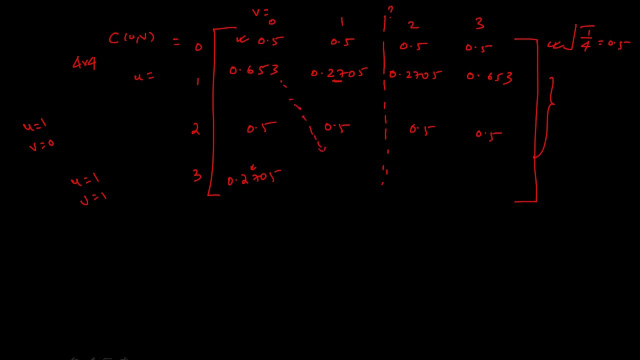 similarly. take this value and shift here, so it would be 0.653. take the mirror again, so 0.653, 0.2705. now let's talk about the sign circle, this term, and in this row, in this row, in this row, the values are negative. so this term is: 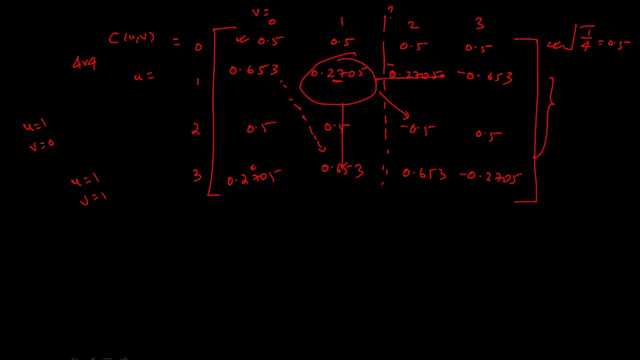 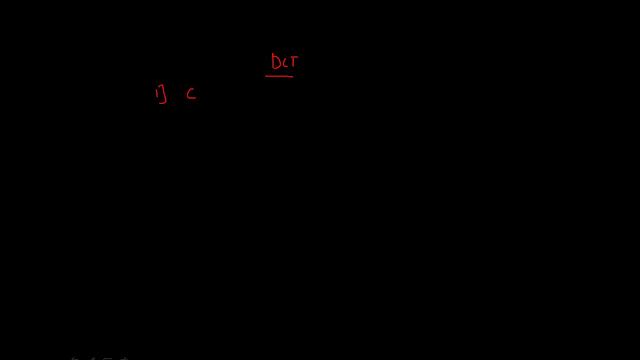 on DCD. the first point is about the cosine transform matrix. the C and the C transpose are not same, so this means it is a, not symmetric matrix. that was the first point. not symmetric matrix. second point is: it is real. as you can see, it was different from DFT when we talk. 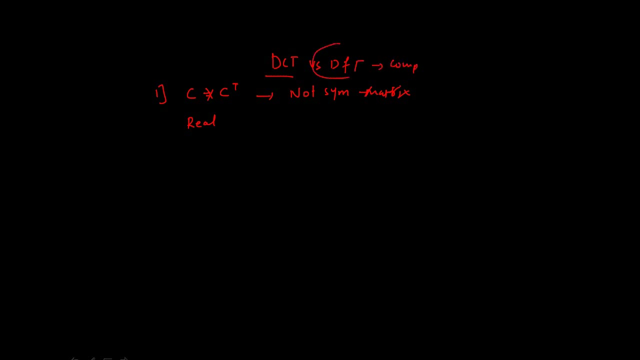 about DCT versus DFT. DFT has the complex terms, but DCT has only the real terms, so it is real and it is orthogonal. that is important. the second point is it is used in JPEG compression. now, this is basically one image compression, so it is. 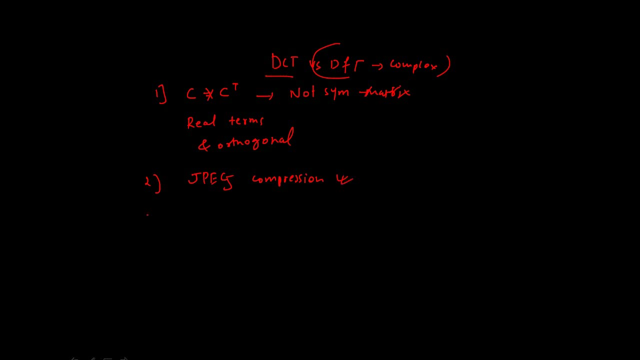 used in image compression. that is the advantage of DCT, and it is also known as the sinusoidal function. this is because we have this cos term and cos looks like this, which is nothing, but you can manipulate in terms of sine, so it is a sinusoidal function.